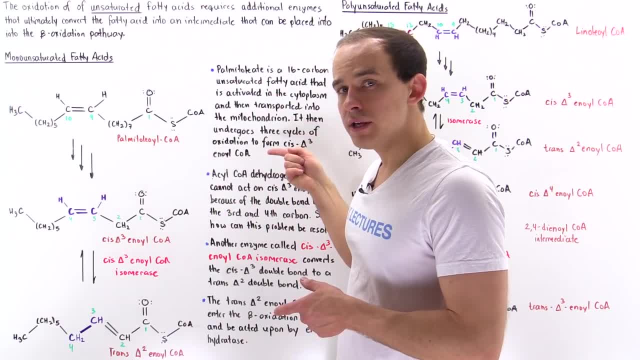 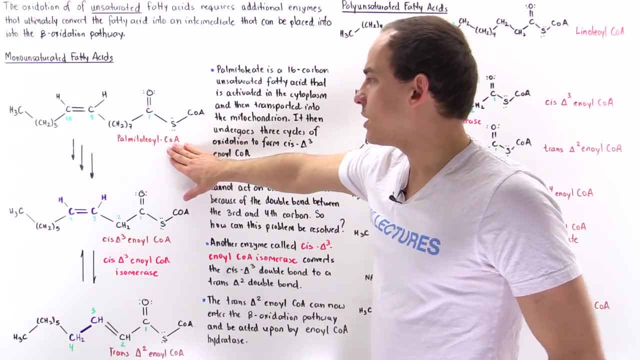 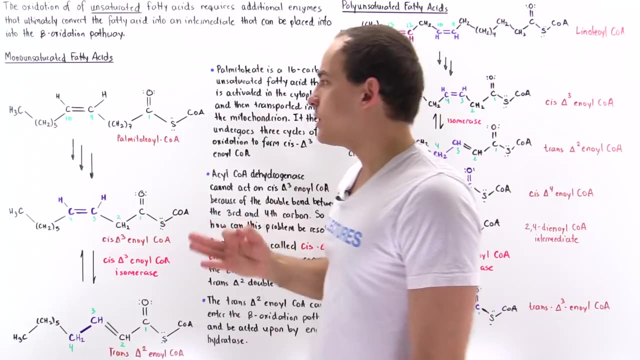 And once we have the active form of the palmitoylate, it then can be transported into the matrix of the mitochondrion. Now, once the palmitoyl coenzyme A is in the matrix of the mitochondrion, it then undergoes three cycles of beta-oxidation, the same beta-oxidation pathway that we discussed in the previous lecture. So once this undergoes three cycles of beta-oxidation, it produces three acetyl coenzyme A molecules and it shortens this 16-carbon molecule into a 10-carbon molecule, this cis-delta-3, in-oil coenzyme A molecule. 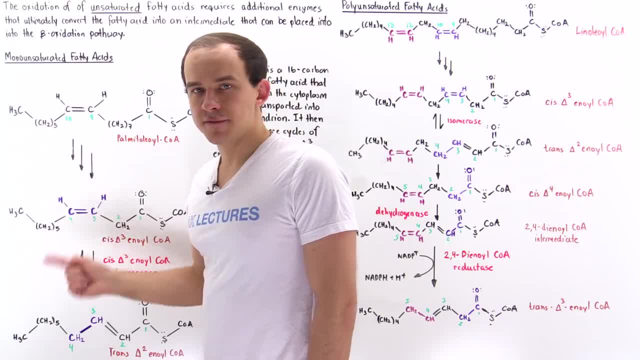 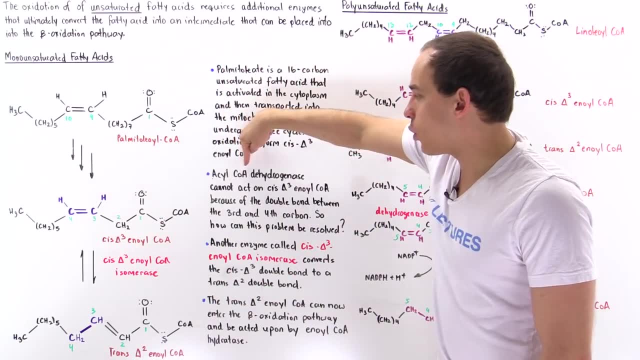 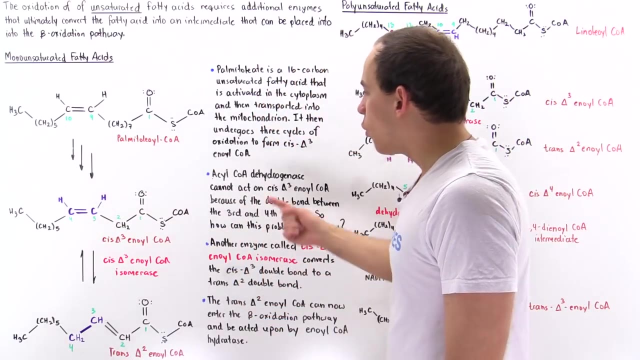 Now, the problem with this molecule is the following: The first enzyme that catalyzes step one of beta-oxidation, the acetyl coenzyme A dehydrogenase, cannot actually act on this molecule. Why Well recall that acetyl coenzyme A dehydrogenase basically generates a double bond. 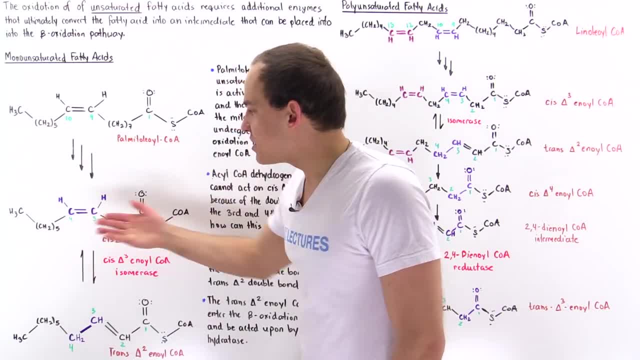 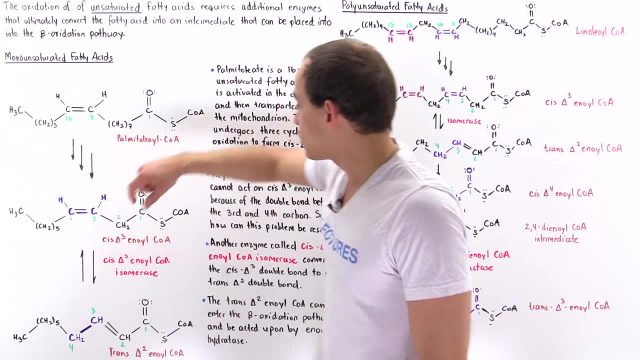 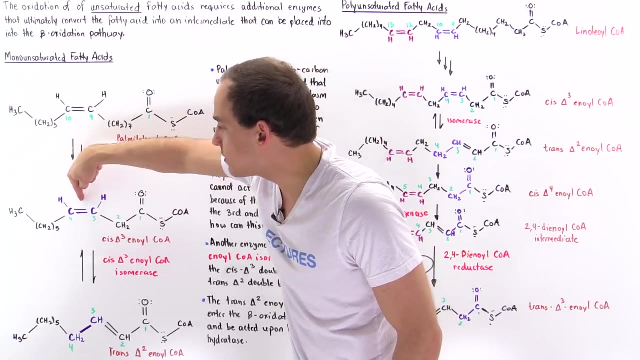 between carbon-2 and carbon-3, and the problem with this molecule is we already have a double bond between carbon-3 and carbon-4, and so this enzyme cannot generate a double bond between carbon-2 and carbon-3 because of the presence of another double bond between carbon-3 and carbon-4. 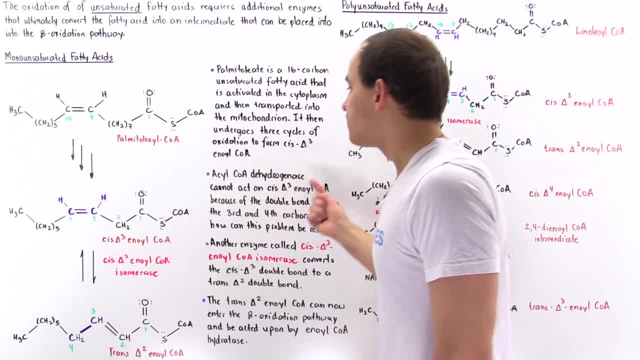 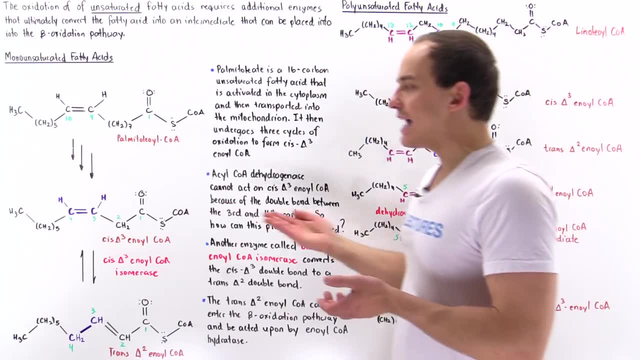 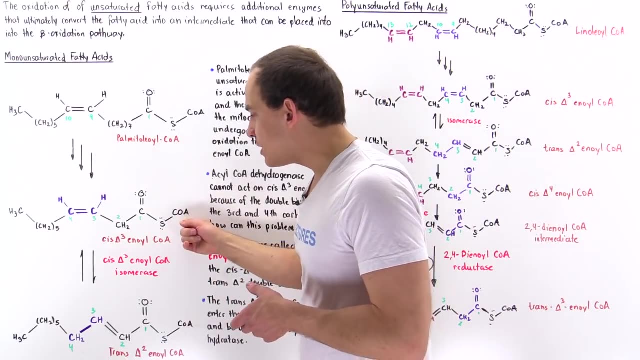 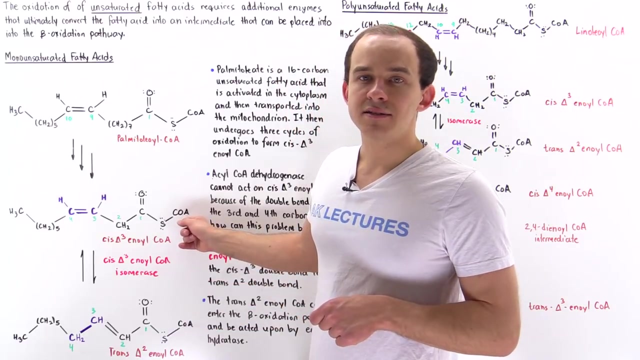 So this molecule is not a substrate for acetyl coenzyme A dehydrogenase. So how exactly do the cells of our body actually prevent this problem, fix this problem? Well, one thing that our cells do is they take this molecule and transform it into an intermediate that can be fed into the beta-oxidation pathway. 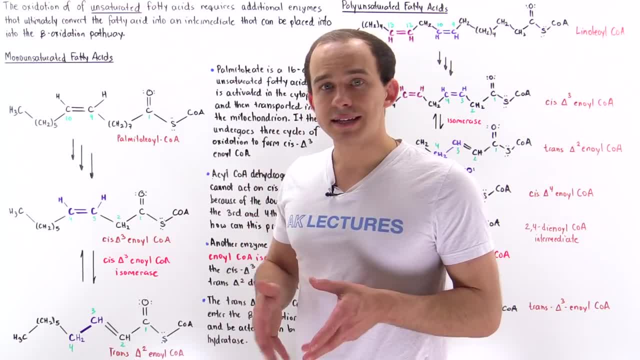 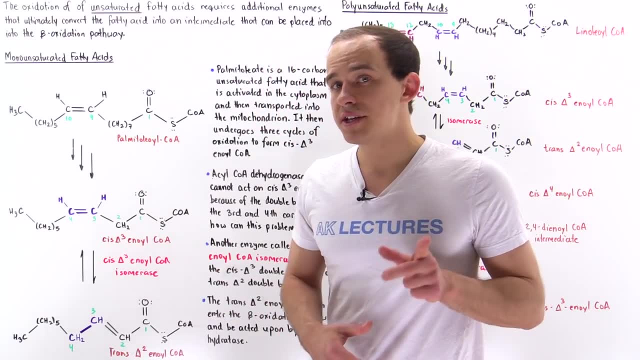 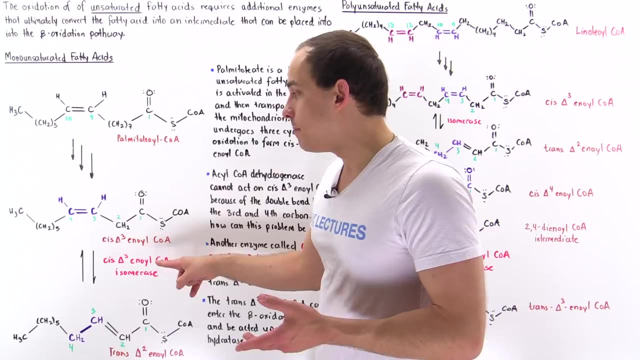 And this enzyme that carries out this process is an isomerase, So it's called cis-delta-3, in-oil coenzyme A isomerase. And what this does is this enzyme changes the location and the configuration of this double bond. 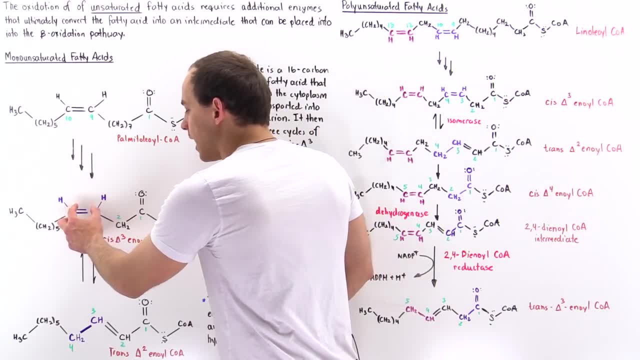 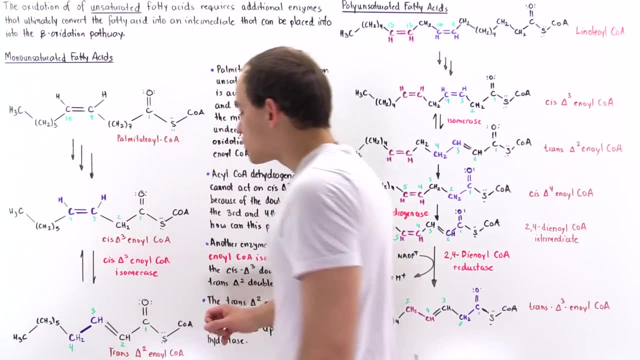 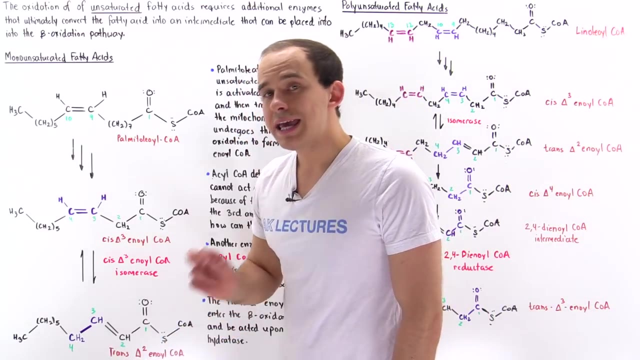 So it takes the double bond and places it onto this position, and that also changes the configuration from cis to trans. So we transform the cis-delta-3, in-oil coenzyme A into a trans-delta-2, in-oil coenzyme A. 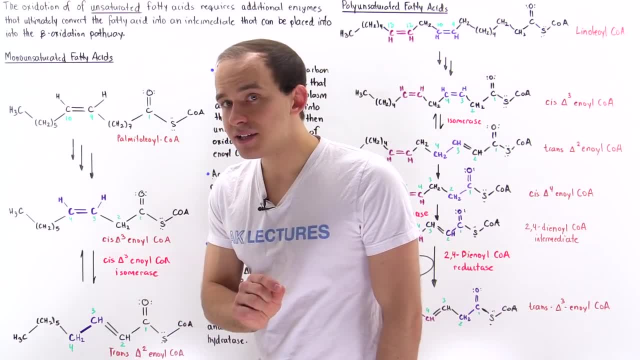 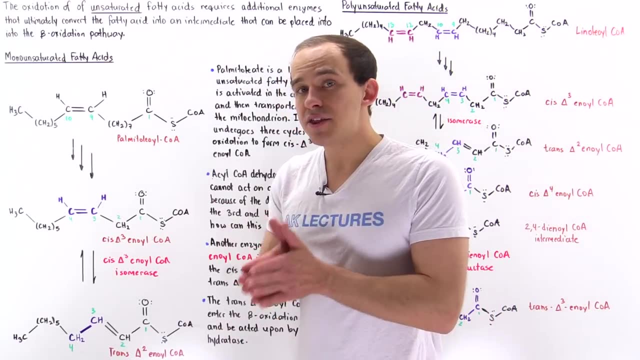 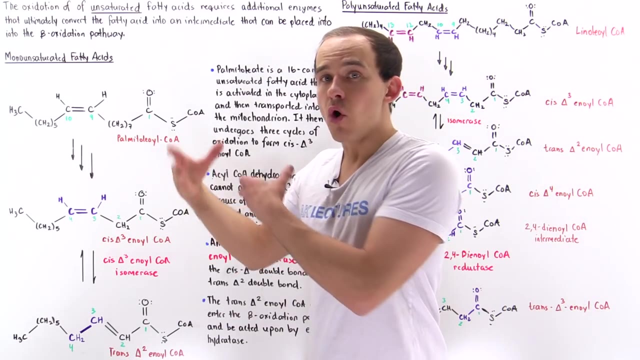 Now this is an important step, because now the second enzyme, namely the in-oil coenzyme A, hydratase in the beta-oxidation pathway can now act on this molecule and then transform it into, ultimately, acetyl coenzyme A. And then we can have three more cycles of beta-oxidation to basically release and produce all those acetyl coenzyme A molecules. So we see that anytime we ingest a fatty acid that contains an odd number of double bonds, this is basically what we're going to find taking place. 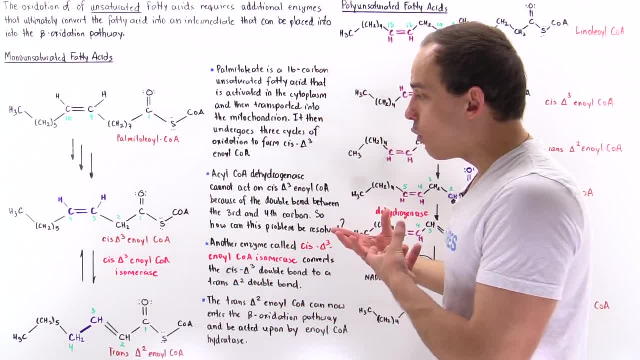 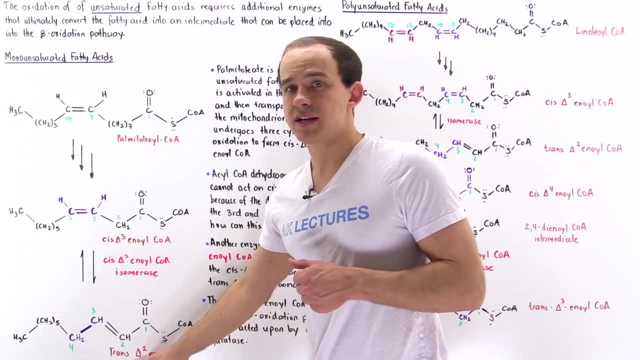 So we're going to have this isomerase that will transform these cis-delta-3, in-oil coenzyme A molecules into the trans-delta-2, in-oil coenzyme A molecules, so that they can be fed into the beta-oxidation pathway. 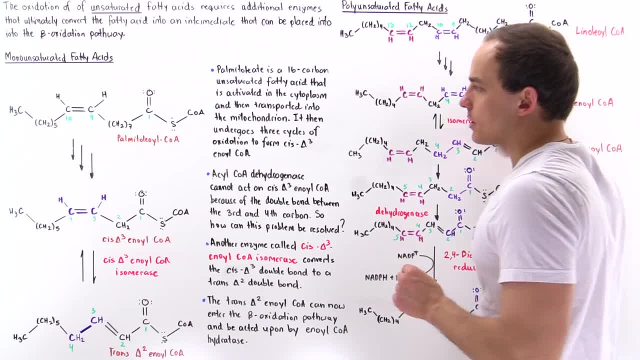 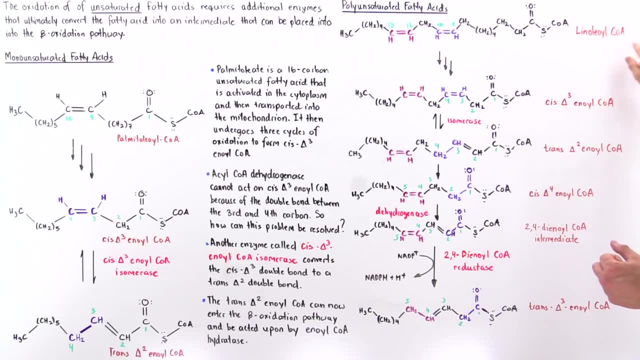 Now what about the case when we have an even number of double bonds in that fatty acid? So to demonstrate what our cells actually do, let's discuss linoleate. Linoleate is an 18-carbon fatty acid that contains two double bonds. 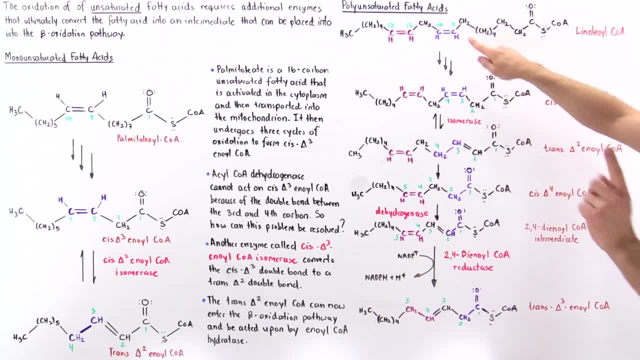 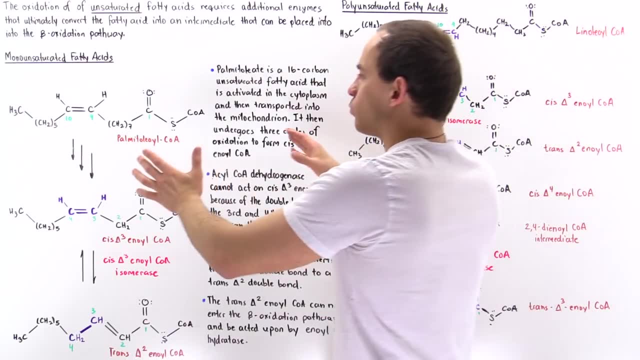 One double bond is between carbon 9 and 10, and the other double bond is between carbon 12 and carbon 13.. Now, in the same exact way that we discussed in this particular case, where we take the palmitoleate, we activate it in the cytoplasm. 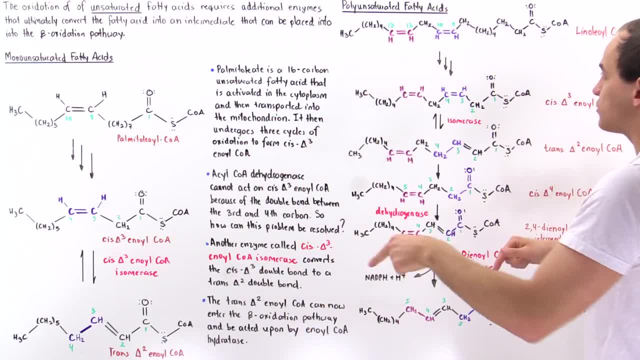 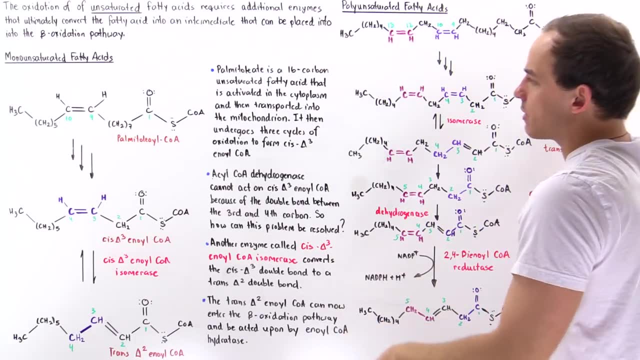 and then move it into the beta-oxidation pathway And then move it into the mitochondria, the matrix of the mitochondrion. The same thing happens here: We take the linoleate, we activate it, we move it into the matrix of the mitochondria of that hepatocyte. 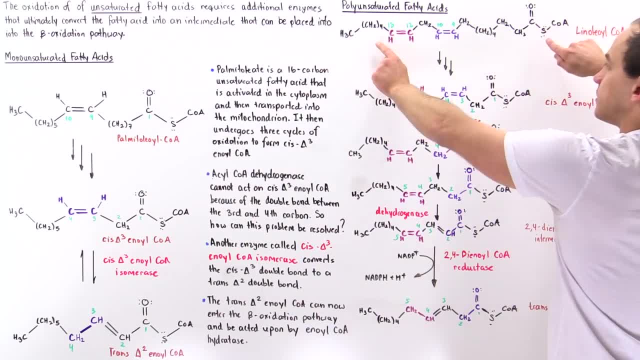 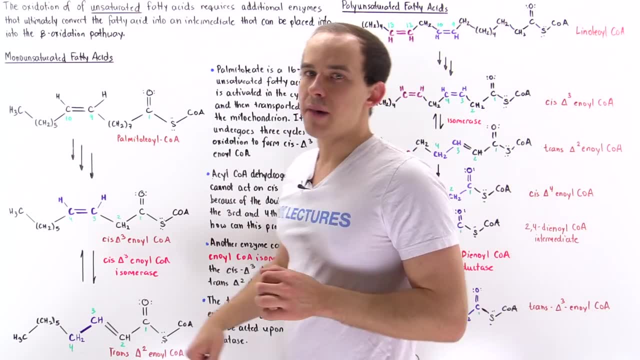 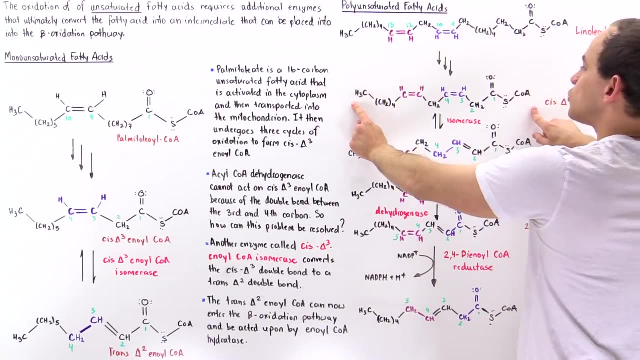 and then, just like in this case, we basically undergo three cycles of beta-oxidation to release three acetyl coenzyme A molecules. So we essentially shorten this 18-carbon molecule to a 12-carbon molecule to form a cis-delta-3 enoyl coenzyme A. 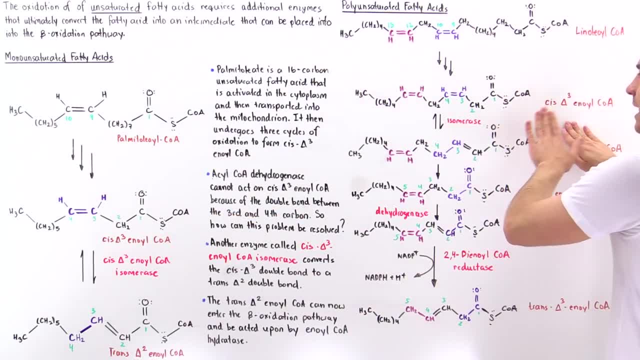 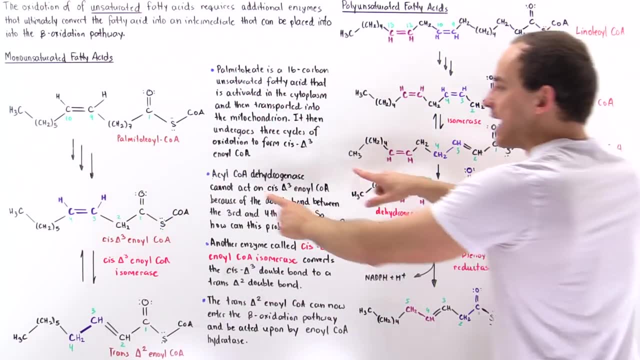 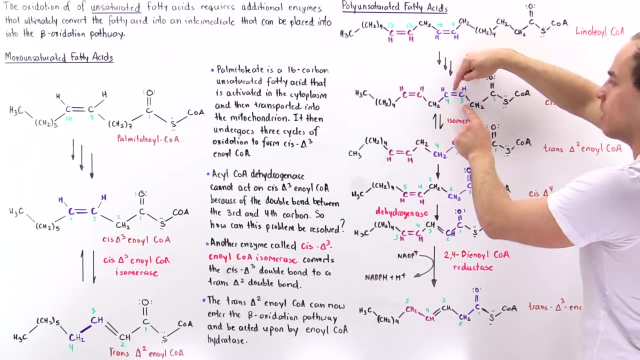 Now notice we basically come to the same exact position as we were in this particular case. So here this acetyl coenzyme A dehydrogenase cannot act on this molecule because of the presence of a double bond between carbon 3 and carbon 4, as we saw in this case. 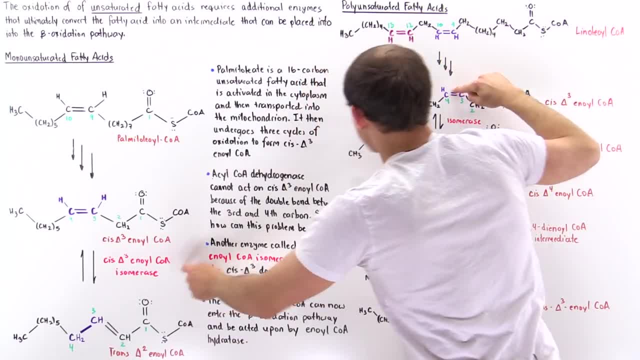 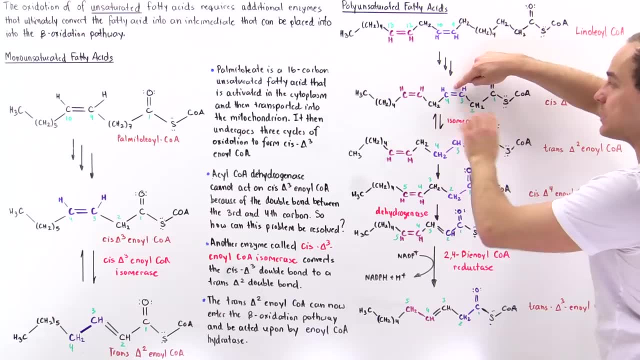 And so, once again, this same isomerase has to act on this molecule to basically change the position and the configuration of this double bond. So we go from a cis-double bond between carbon 3 and carbon 4. to a trans-double bond between carbon 2 and carbon 3.. 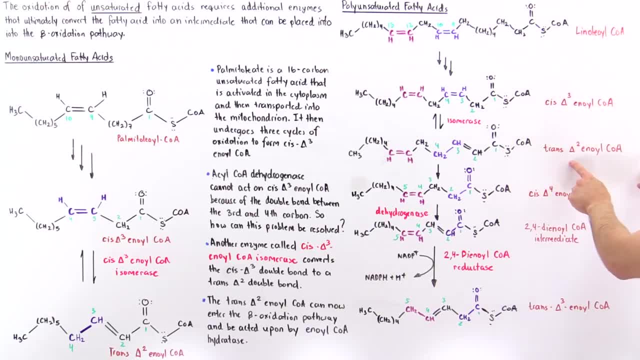 And so once we form this intermediate, this is a trans-delta-2 enoyl coenzyme A, as we saw in this particular case. now this can basically complete that beta-oxidation pathway to basically form a cis-delta-4 enoyl coenzyme A molecule. 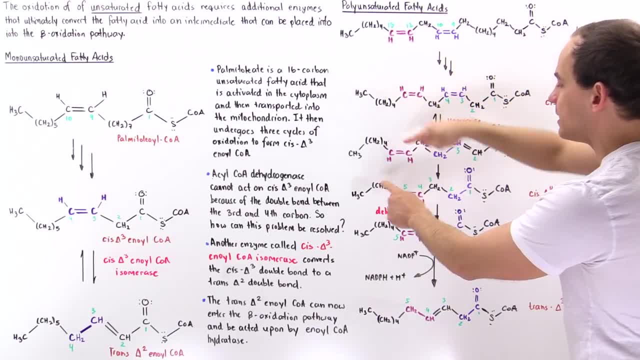 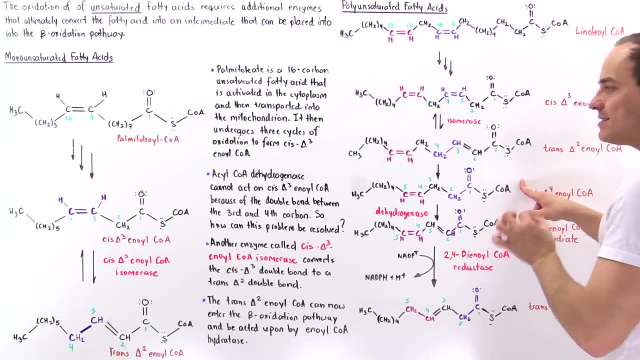 that now contains only one double bond, as can be seen, between the carbon 4 and carbon 5.. Now this molecule is a substrate to acetyl coenzyme A dehydrogenase, And once the acetyl coenzyme A dehydrogenase acts, 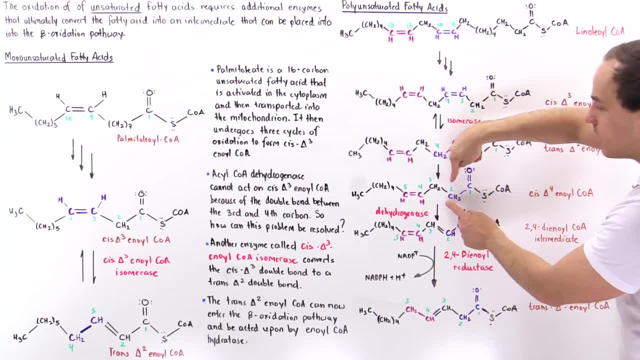 on this molecule. it forms a double bond between carbon 2 and carbon 3.. And so we form this molecule, which we call the 2,4-di-enoyl coenzyme, A intermediate. Now, the problem with this molecule is: 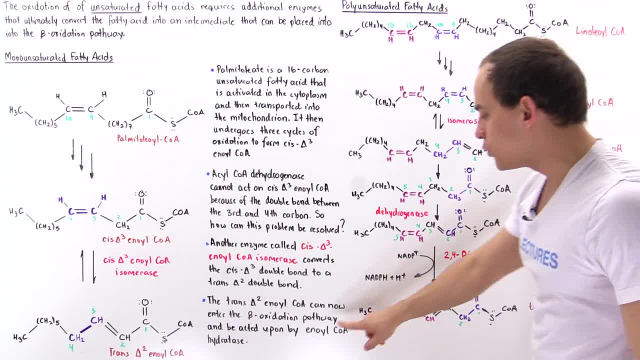 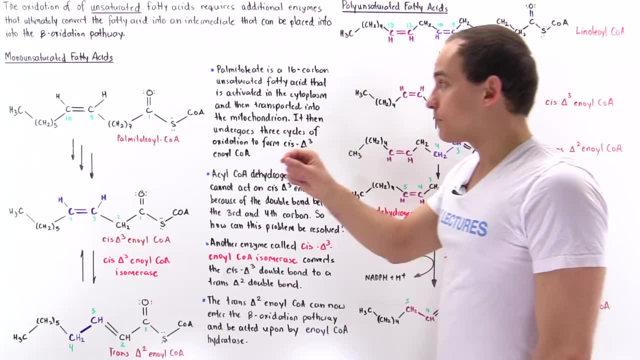 this molecule is not a substrate molecule to enoyl coenzyme A hydratase. So enoyl coenzyme A hydratase, the second enzyme in the beta-oxidation pathway, cannot actually act on this molecule. 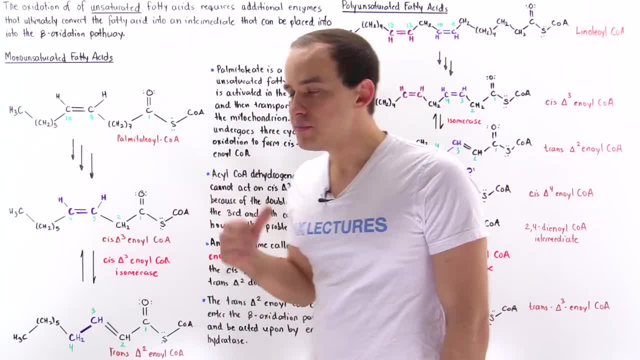 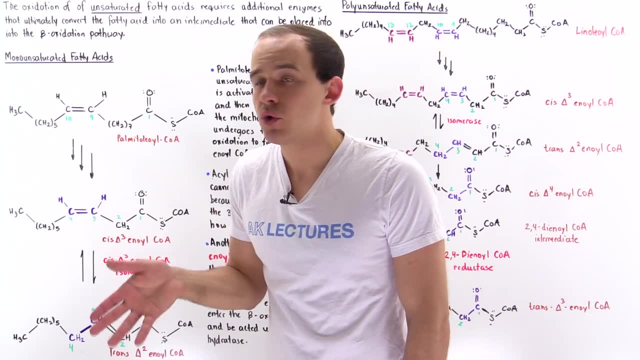 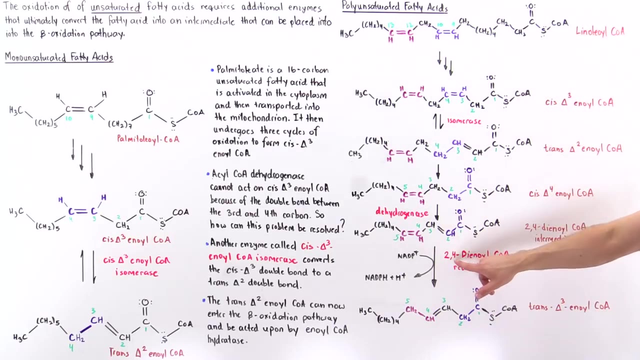 And so, once again, we have to use some type of enzyme to basically transform this molecule into a molecule that can ultimately be fed, can be incorporated into the beta-oxidation pathway, And the enzyme that carries out this process is known as 2,4-di-enoyl coenzyme A reductase. 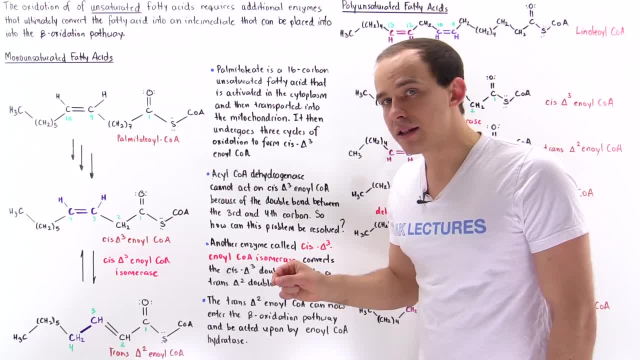 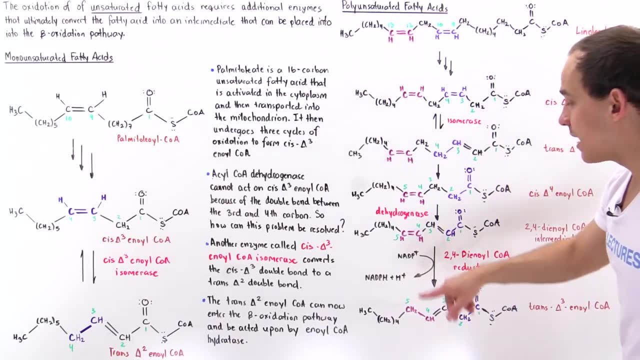 It basically uses an NADP-plus molecule to basically oxidize this intermediate into this molecule, at the same time reducing and forming the NADPH. Now, once we form this molecule, a trans-delta-3 enoyl coenzyme A, 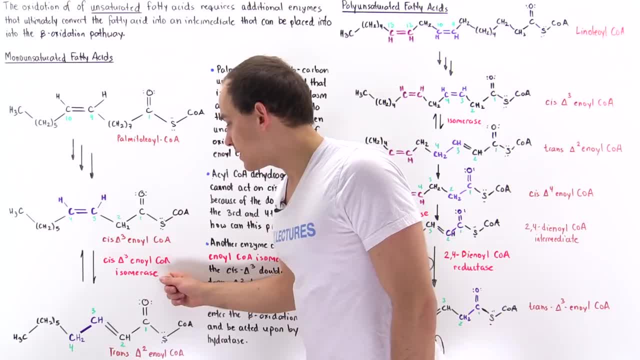 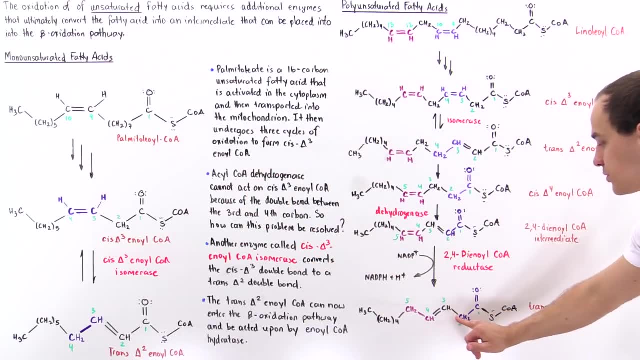 now an isomerase. this isomerase here can act on this molecule, basically move that double bond onto this location here. So if the isomerase acts on this molecule it will form an intermediate. that is not shown here. 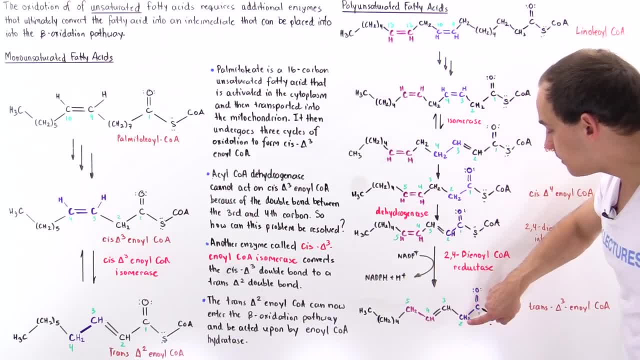 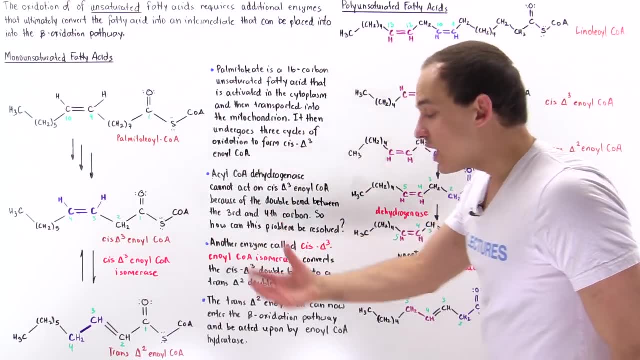 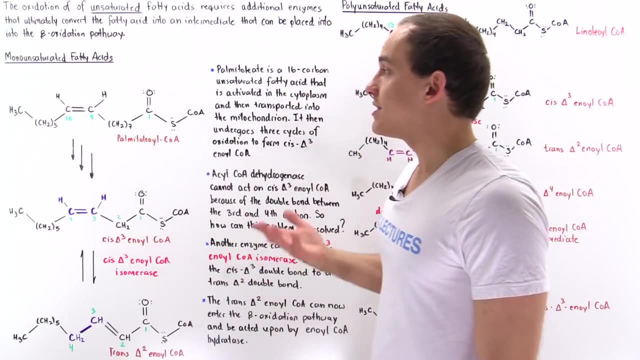 but that intermediate will basically have a double bond between carbon-2 and carbon-3.. and then that can be fed into the beta-oxidation pathway and ultimately this entire fatty acid can be broken down into acetyl coenzyme A molecules. 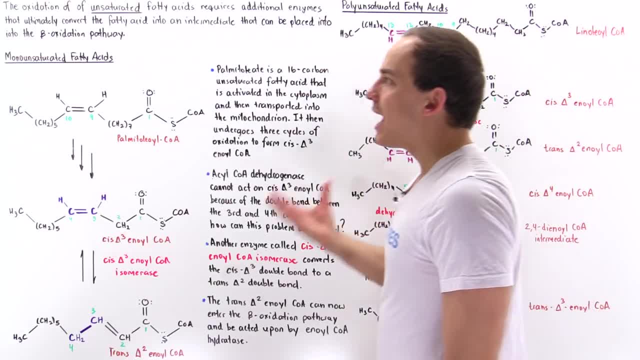 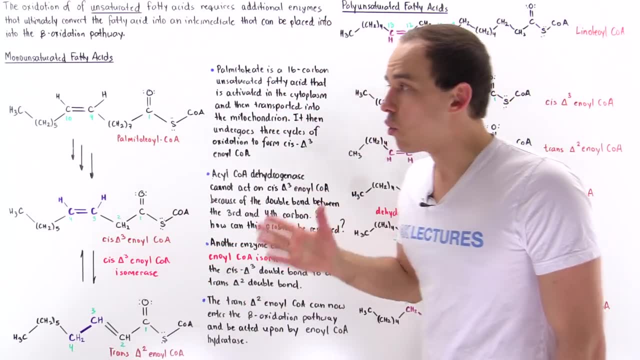 So we see that, no matter what type of unsaturated fatty acid that we actually ingest, if it contains either an odd number of double bonds or an even number of double bonds, we see that our cells can use an isomerase. 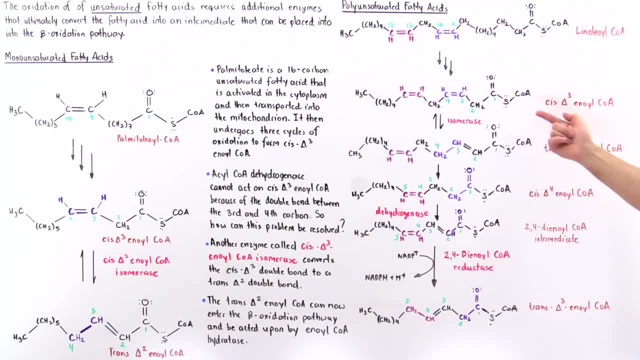 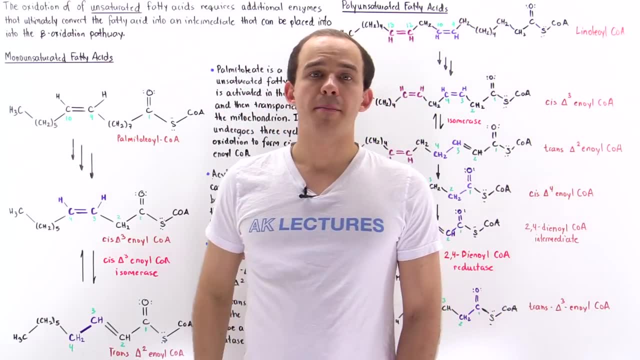 or, in this case, the combination of an isomerase and a reductase to basically transform and break down those fatty acids into acetyl coenzyme, A molecules. 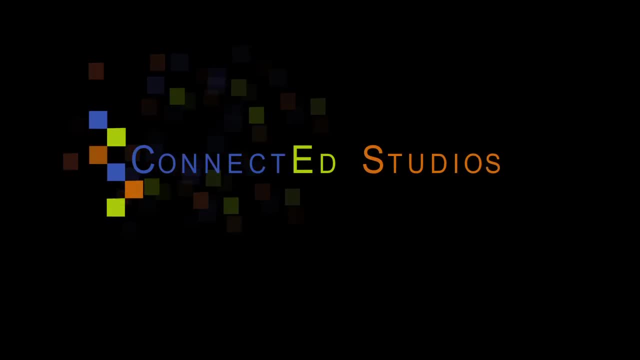 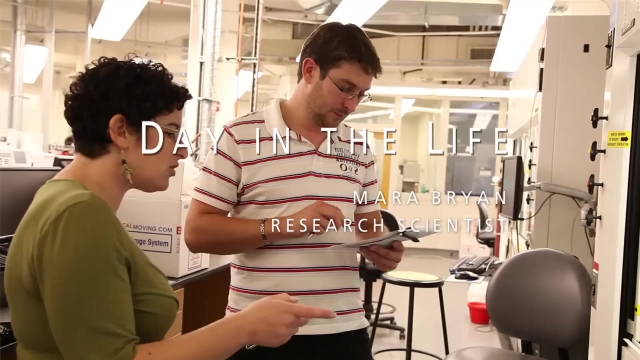 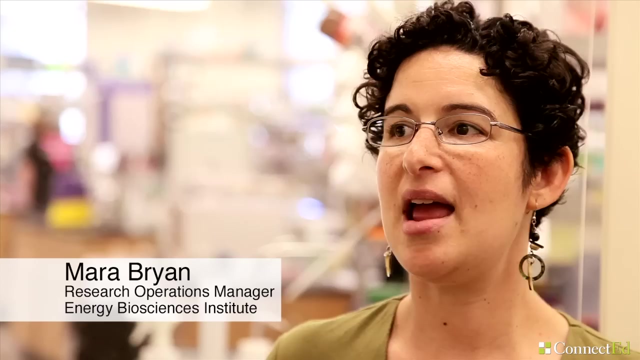 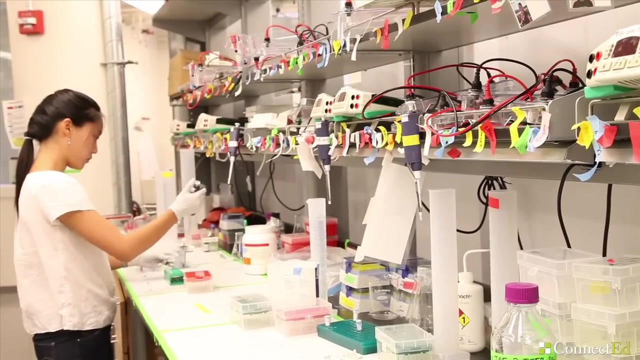 I'm Mara Bryan. I'm the research operations manager at EBI. EBI is the Energy Biosciences Institute and it was formed to apply the techniques and knowledge in modern biology to problems in energy. The work being done on EBI is important because we're taking a big-picture approach to the problem. If 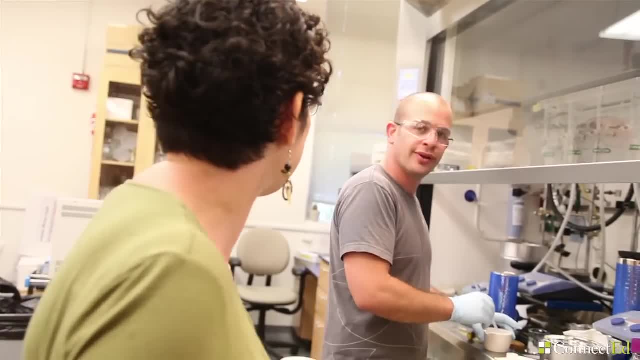 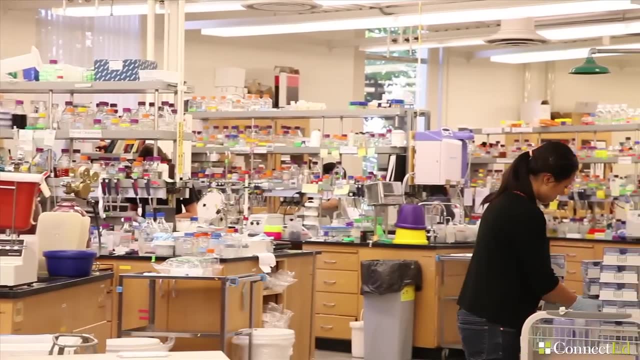 it's being done environmentally sustainably, if it's being done economically sustainably and socially sustainably. So we're looking at a big-picture version of a problem that affects many, many people. I'm responsible for the day-to-day operations of the lab and making sure that the research here 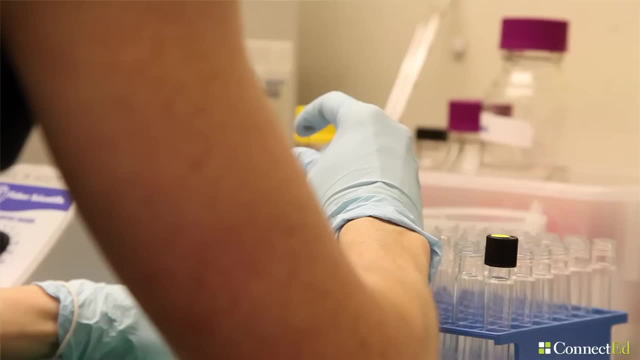 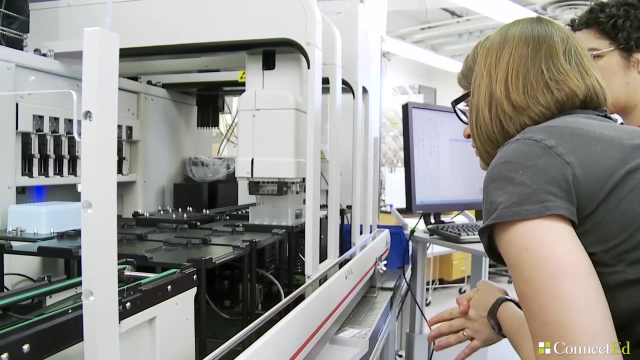 happens. So that means I'm in charge of making sure the researchers have the supplies they need, making sure that all the instruments are functioning, making sure that everything's organized. A lot of it is people skills in making sure that people are doing things the way they're supposed to be.